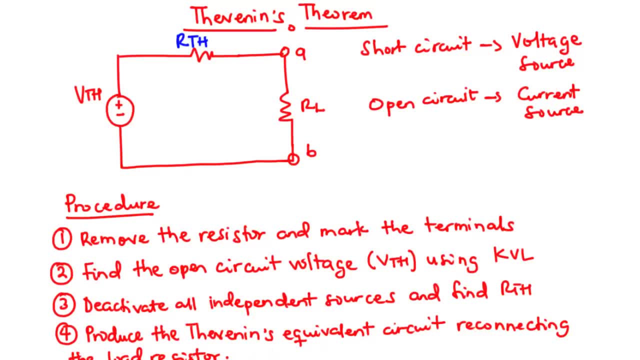 In today's video we are going to study the concept and application of Thevenin's Theorem. We are going to learn how to find the Vth, Rth and the current flowing through a particular resistor. Now, if you are new here, make sure you subscribe to this channel. 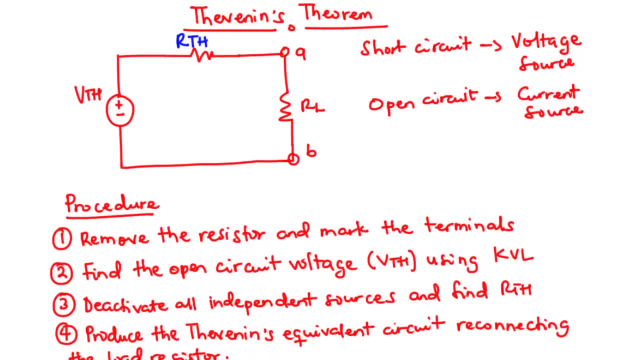 like this video and share this video to all your friends. So, without wasting much time, let's get into today's lesson. So, according to Thevenin's Theorem, any linear circuit connected between two terminals can be replaced by a Thevenin's voltage in series with a Thevenin's resistance. 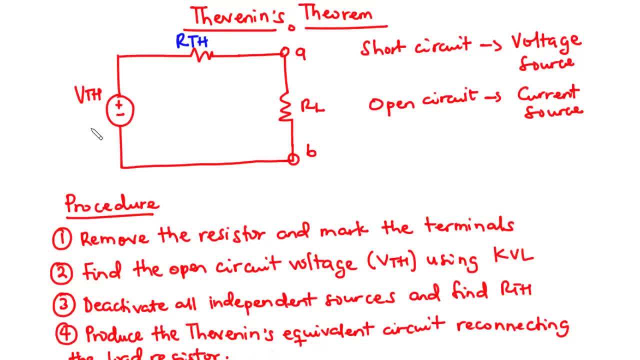 So the Thevenin's voltage, that is, Vth, is the voltage seen between the two terminals AB, And the Thevenin's resistance, Rth, is the equivalent resistance seen between the two terminals when all the independent sources are used. 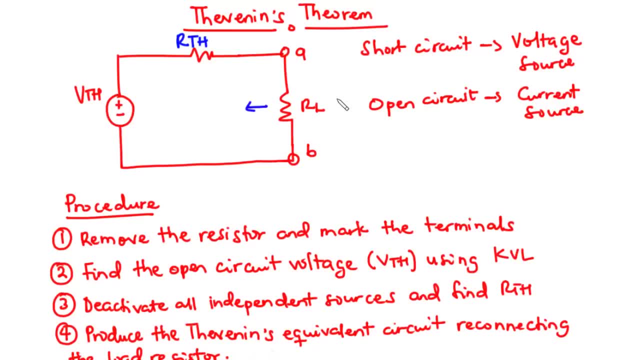 The current going through the terminal is Rd-activated or D-activated, And we also have RL, which is called the load resistance. Now this load resistance is in series with Rth, so that the current produced by Vth will be the same current flowing through Rth and then RL. 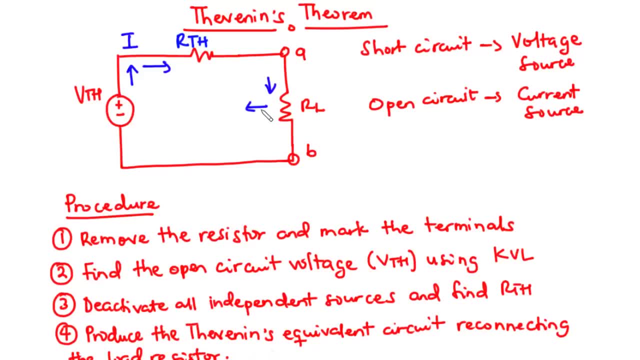 This RL is also the resistance you want to find the current flowing through, flowing through the load resistor, then that is given by. I equals the voltage divided by the total resistance of the circuits. Now, since these two resistors are connected in series, then RT is equal to the sum of these two. Now, since we have V to be Vth, we say that I is equal. 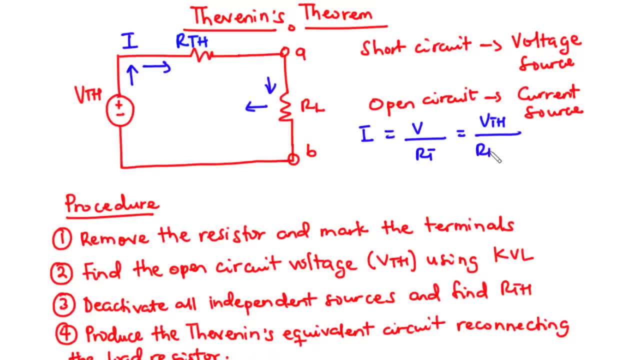 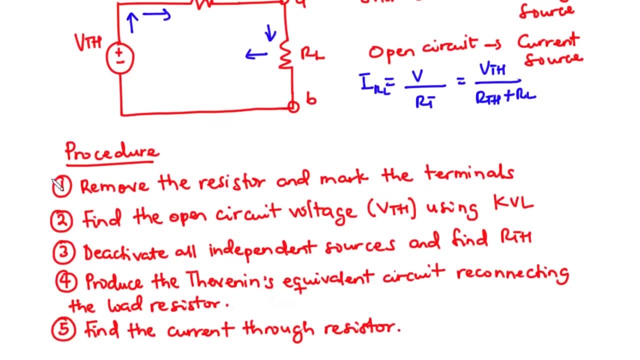 to Vth divided by Rth plus RL. So basically, this is how to find the current flowing through the load resistor. So how do we even arrive at the values of Vth, Rth and then RL Now? to do so, we are going to use the steps outlined below. So, given any linear network connected between 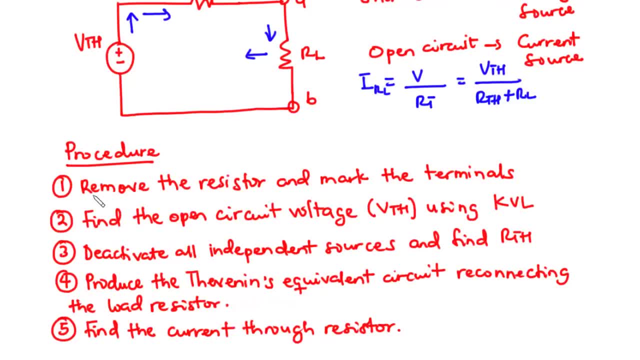 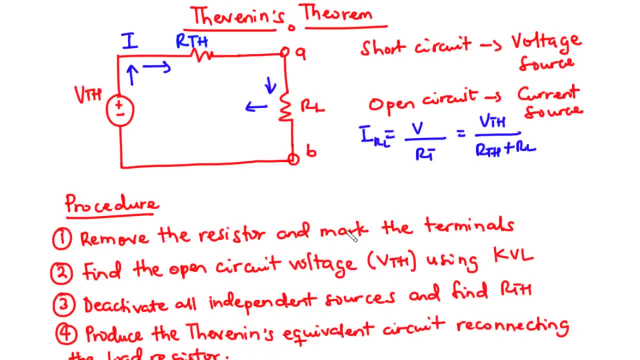 two terminals. the first thing we need to do is to remove the resistor which we want to find the current flowing through, and then mark the terminals. Secondly, we need to find the open circuit voltage, that is, Vth, using the Kirchoff's voltage law, and then, thirdly, we want to deactivate all the independent sources and 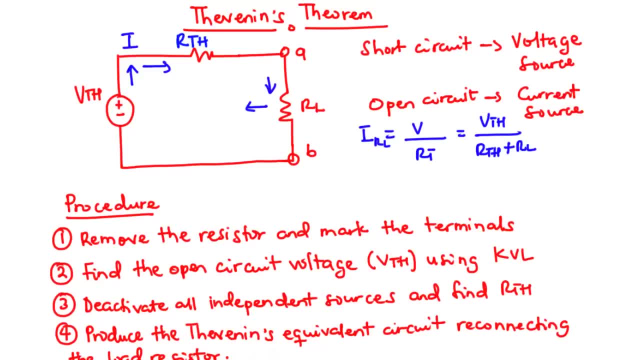 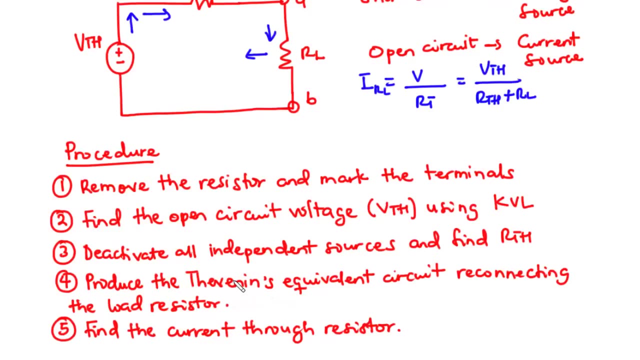 find Rth. So in deactivating the independent sources, we are going to short circuit all voltage sources and then open circuit all current sources. Next, we are going to produce the Thevenin's equivalent circuits reconnecting the load resistor. So this is the Thevenin's equivalent circuit with the load resistor reconnected. 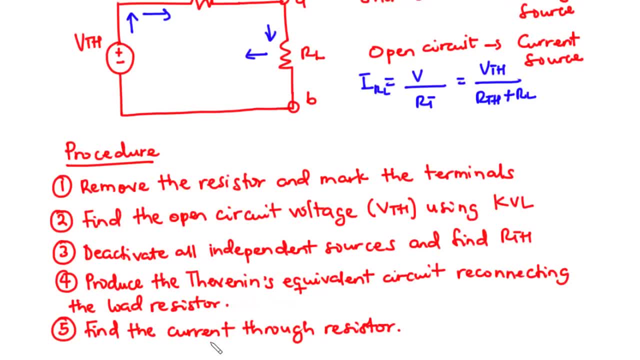 And then, lastly, we are going to find the current through the load resistor. that is, using the formula I equals Vth divided by Rth plus RL. So, basically, these are the various steps we are going to use to to find Vth, Rth and the current flowing through a particular resistor. 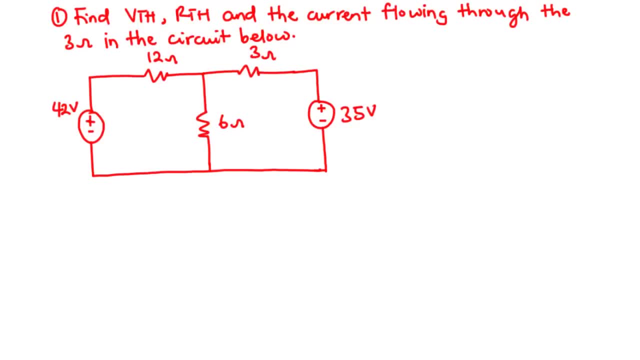 Now let's take a few examples. Now let's take the first example. Find Vth, Rth and the current flowing through the 3 ohms resistor in the circuit below. So for this circuit we have 2 voltage sources: 42V and then 35V. 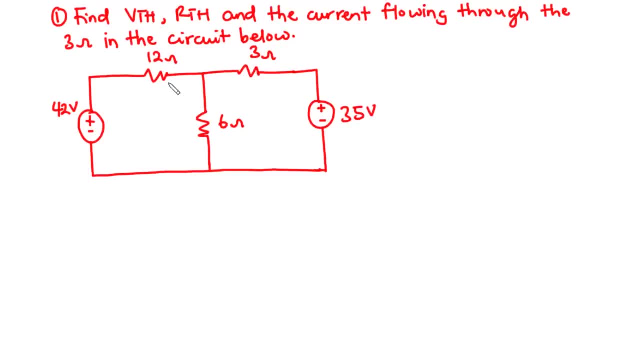 And then we have 3 resistors connected in the circuit. We have the 12 ohms, 3 ohms and the 6 ohms. Now we are going to find Vth, Rth and the current flowing through the 3 ohms resistor. 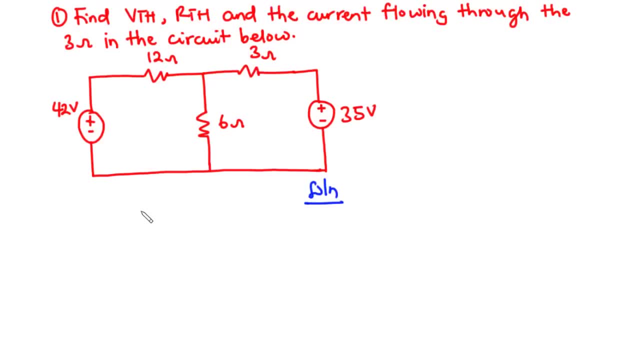 Now to solve this circuit using Thevenin's theorem, the first thing we need to do is to remove the resistor. we want to find the current flowing through, And then we mark the terminals and then find Vth. So let's do that together. 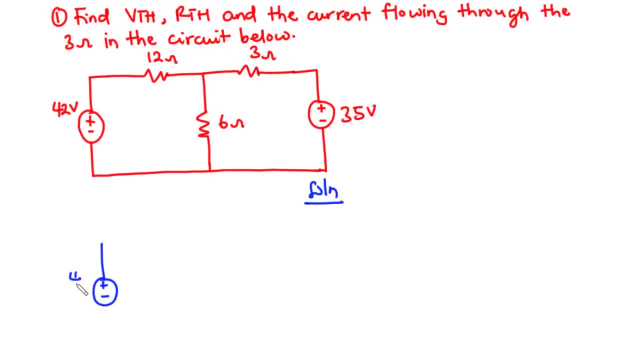 Ok, So we have the voltage source, that is 42V, We have this resistor to be 12 ohms, We have this to be 6 ohms And then we are going to remove the 3 ohms resistor. We mark the terminals AB. 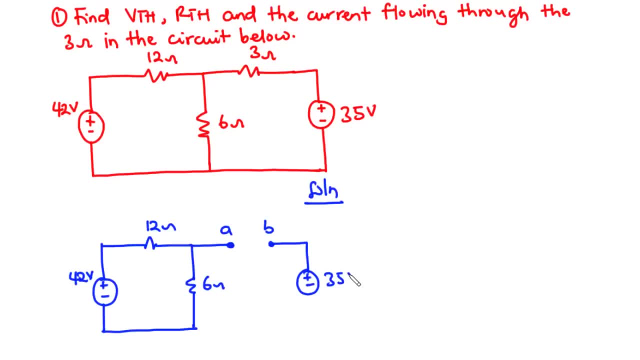 We have the 35V source, We have the 45V to be 7 ohms, We have the 30V to be 32 Ohms And then we are going to complete the circuit. So we call this Vth. 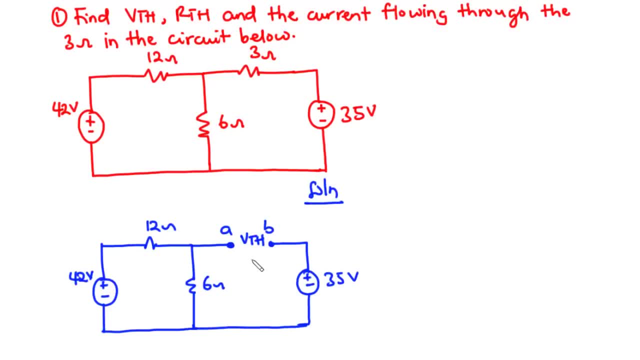 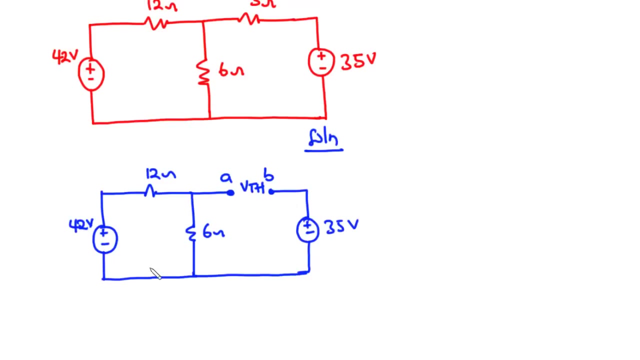 That is the open circuit voltage seen between the 2 terminals. So at this point we are going to distribute current in the circuit and then we move on to find the value of Vth. So for this circuit we have 2 loops. Let's call this loop1.. 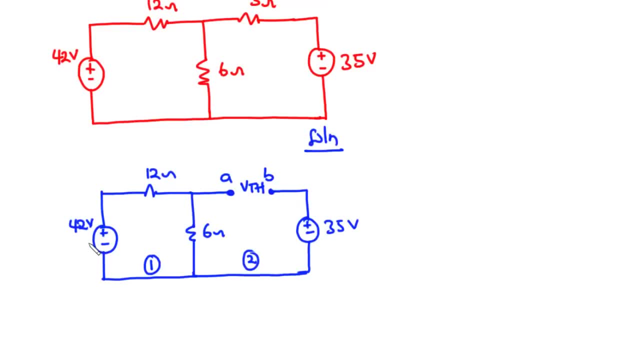 And then loop2.. Now this 42V drives current. This way we have 2 loops And then loop 1. in the clockwise direction, that is, considering the conventional flow of current. Now let's call this current I. So the current I produced by the 42V is the same current that flows through the 12 ohms. 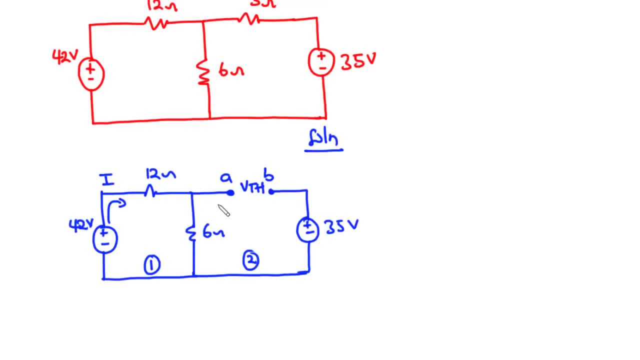 resistor and the 6 ohms resistor. Now, because we have an open circuit here, no current will flow in this direction. The current that flows through the 12 ohms resistor will flow through the 6 ohms resistor and return to the negative terminal of the voltage source. 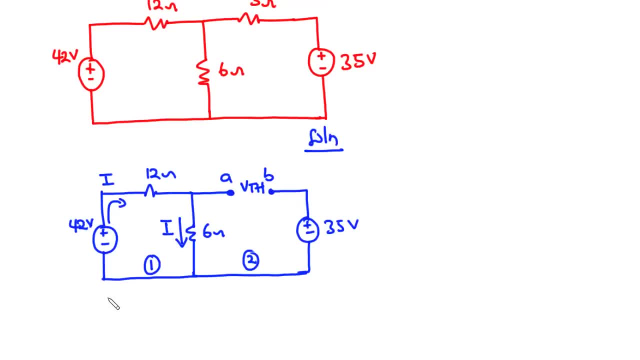 Therefore, we can find the value of I produced by the 42V. Now, since the same current flows through these two resistors, it means that they are connected in series. Therefore, we have I to be equal to V divided by RT. We have the value of V to be 42.. 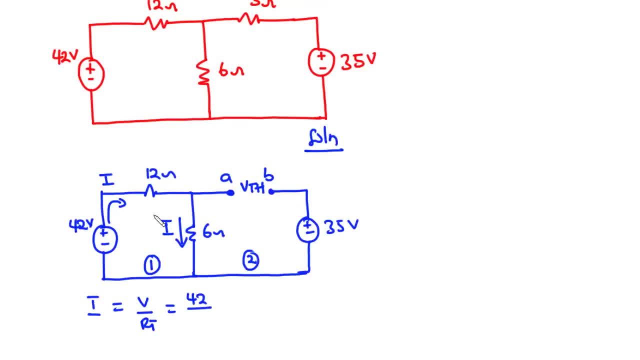 So 42 divided by we are going to add these two values, 12 plus 6 is 18.. And this is equal to 21 over 9.. So we have the current I to be 21 over 9A. Now, since we have the value of I, we can generate an expression for Vth and find the. 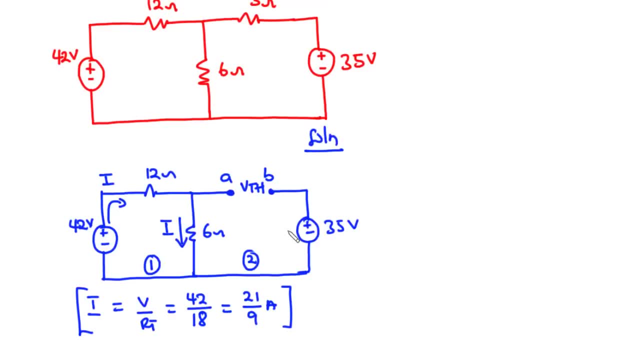 value of Vth. So to find the value of Vth, we are going to use the second loop. Now let's choose any arbitrary direction for Vth. Now, this is Vth. here it will be dust, And this is least. 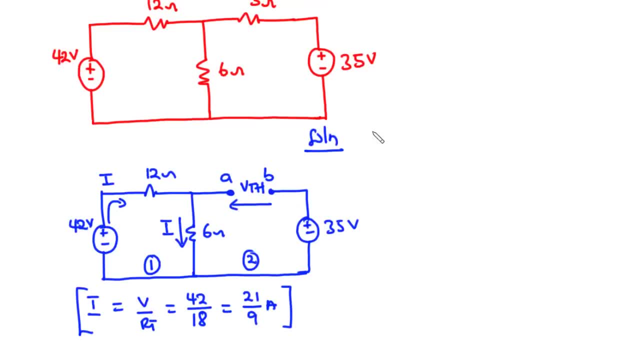 So we are going to move in the anti-clockwise direction. So still considering the second loop and then taking the anti-clockwise direction for the 35 voltage source, then we say that 35 plus Vth, because Vth is also in the same direction as the 35 volts. 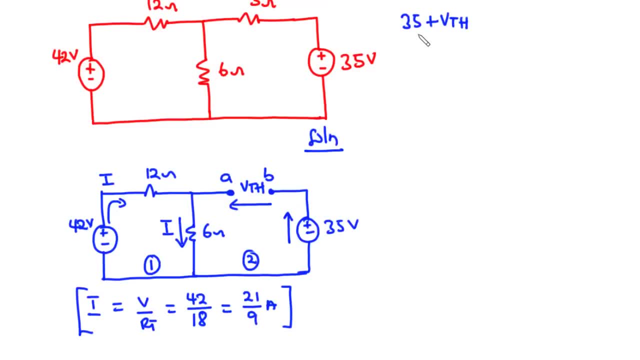 They are all directed anti-clockwise. So we have 35 plus Vth equals the sum of the voltages dropped across the loop. So we have I times 6, also moving in the anti-clockwise direction. So that is equal to 6 times I. 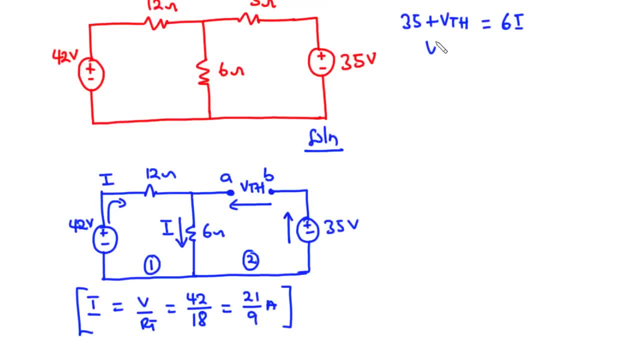 Now, since we want to find the value of Vth, we are going to transpose 35 to the right hand side, So this becomes 6I minus 35.. We know the value of I to be 21 over 9.. So that is 6 times 21 over 9 minus 35. 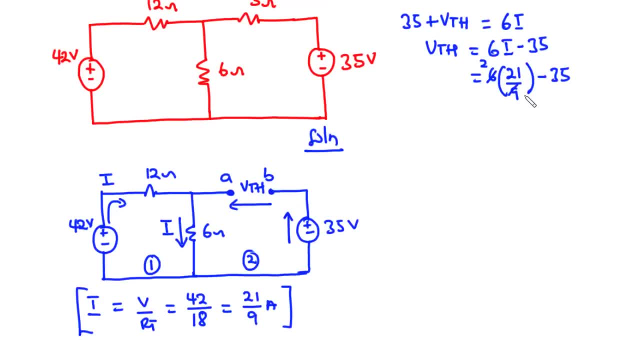 3 goes into 6 two times. 3 goes into 9. three times We have 2 times 21, which is 42.. 42 divided by 3 is 14.. So we have 14 minus 35 and that is equal to negative 21.. 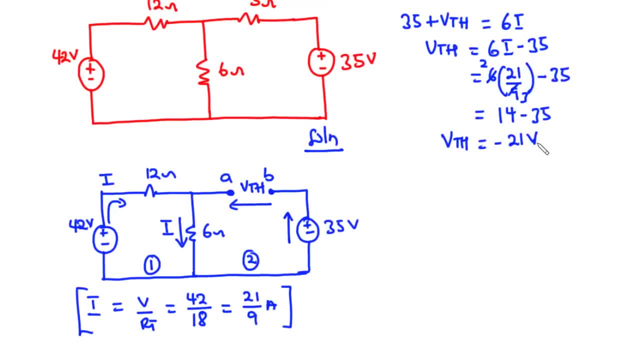 Therefore, we have Vth to be negative. Next, we are going to find the value of Rth. So let's redraw this circuit, deactivating all the independent sources. Because we have voltage sources, we are going to short-circuit them. 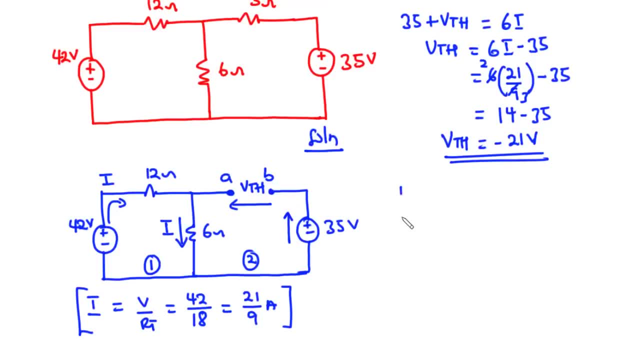 So the circuit becomes. So we have the 42 volts being short-circuited, We have this to be the 12 ohms resistor, The 6 ohms resistor. We have the terminal AB. We have the 12 ohms resistor. 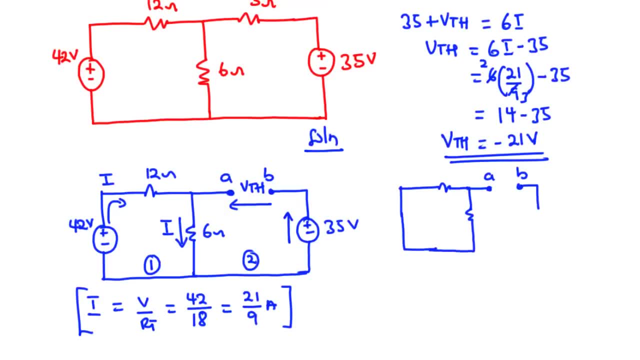 The 35 volts is also short-circuited. And then we want to find the value of Rth, That is, the equivalent resistance seen between the two terminals. Now we said in the previous lessons that when you go through a loop without passing through any other circuit element except two resistors, 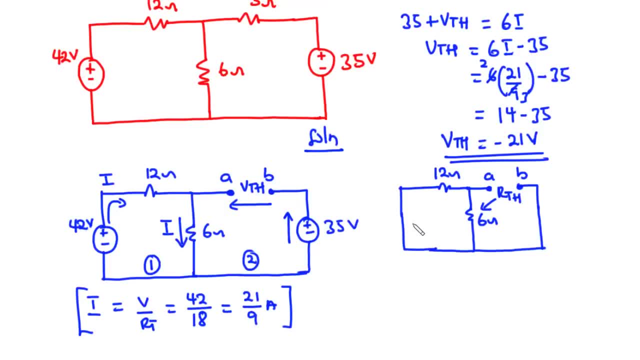 then it means that the two resistors are connected in parallel. So we see this case here, where we go through this loop without passing through any other circuit element except these two resistors. Therefore we say that these two resistors are connected in parallel. 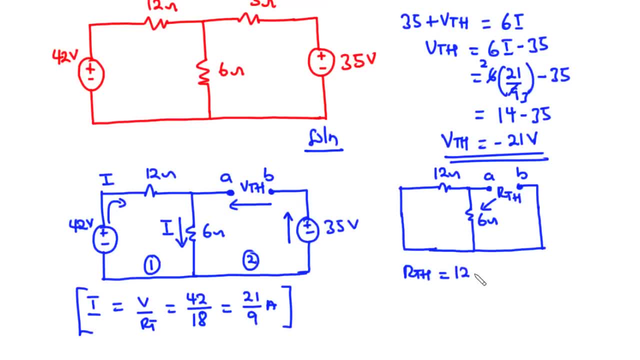 Therefore, Rth is equal to 12 parallel 6, and this is equal to 12 times 6 divided by 12 plus 6.. 12 times 6 is 72.. 12 plus 6 is 18.. So 72 divided by 18 is equal to 4.. 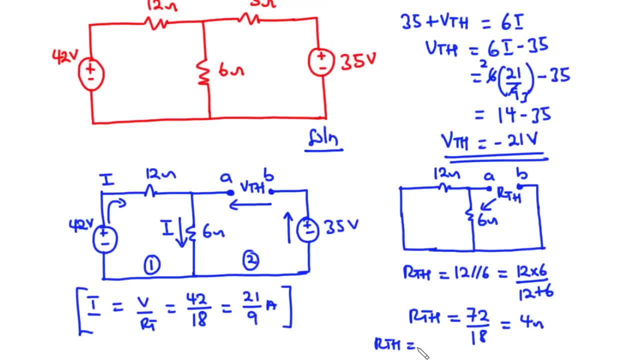 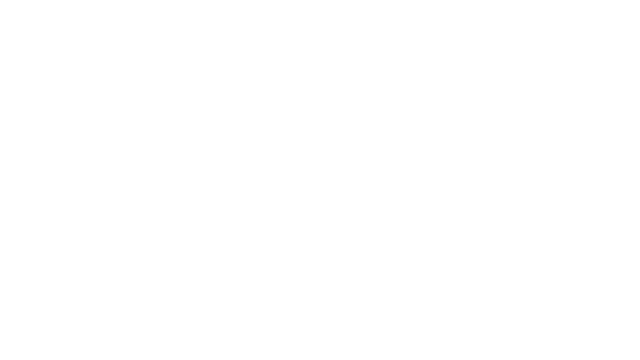 Therefore we have Rth to be 4 ohms. Now, since we have the value of Vth and then Rth, let's find the value of the current flowing through the 3 ohms resistor. So for the 7 ohms equivalent circuit, we have Vth. 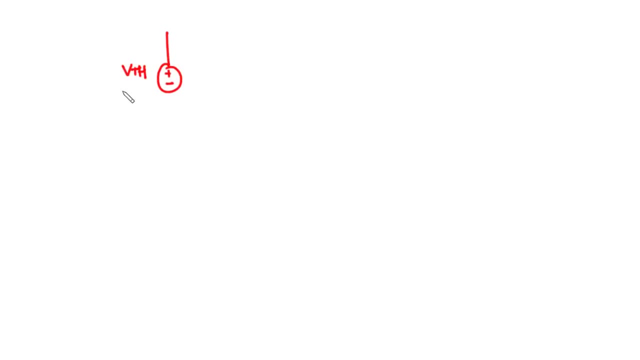 And then Rth. This component is somewhat similar to the current of Rth, So from here on we say that the current of Cis is negative Rth and Rth is reported to be negative 21 volts connected in series with Rth. 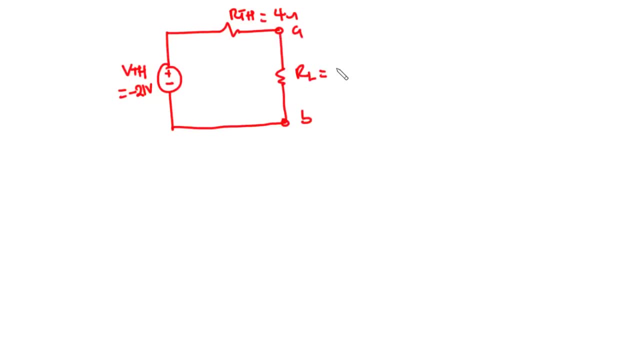 Which was found to be 4ohms, And then, since we want to find a current flowing through the 3 ohms resistor, we are going to connect the 3 ohms resistor between the two terminals. So that is the load resistance: 3 ohms. 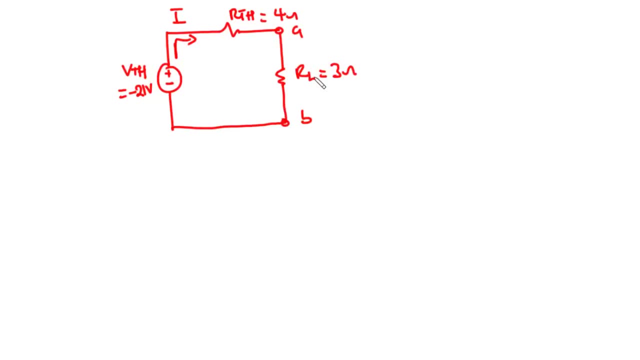 circuits and if you want to find the current flowing through the load resistor, which is the three ohms resistor, that is equal to vth divided by rth plus rl. now, the reason why we are going to add these two resistor values is that these two resistors are connected in series. now we have vth. 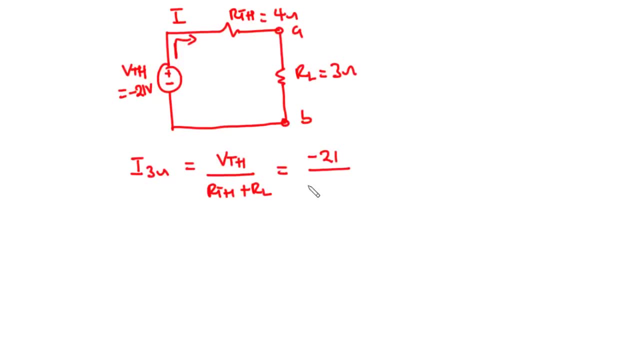 to be negative 21 divided by rth4 plus rl3, this becomes negative 21 divided by 7. therefore, we say that the current flowing through the three ohms resistor is equal to negative three amperes. now let's take the next example. now for the previous example. we had two voltage sources in this example. 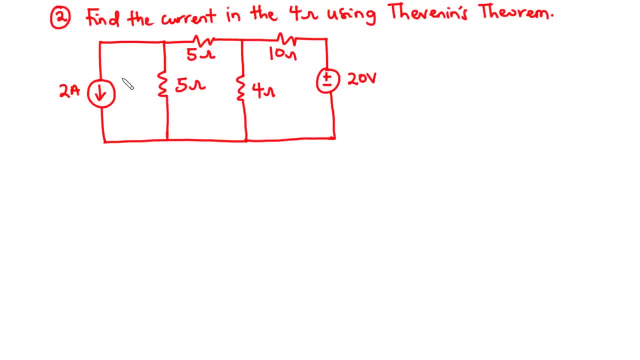 we have one voltage source and one current source. Now let's find the current flowing through the 4 ohms resistor using Thevenin's theorem. Now the first thing we need to do is to remove the 4 ohms resistor, That is. 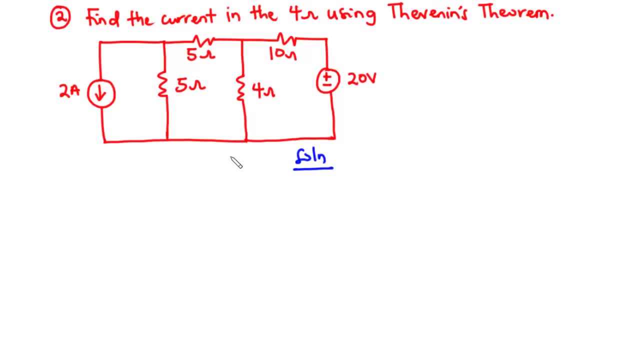 the resistor. you want to find the current flowing through, Mark the terminals and find Vth. So let's do that. So, after drawing this circuit, let's consider this particular loop Now. for this loop, we have an independent current source. Now what this is going to do is this independent current source is to 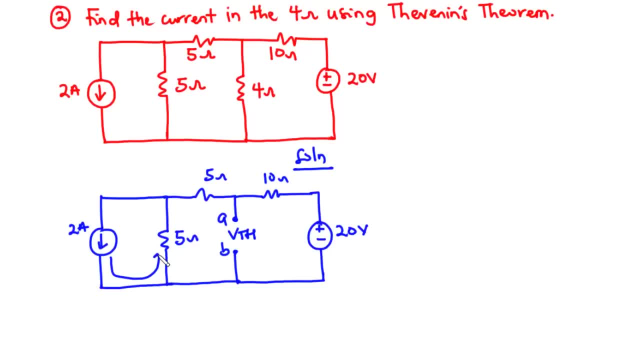 flow in the anticlockwise direction, circulating in this loop over and over. So we have the 2 amperes current source. Now let's consider this particular loop. Now, for this loop, we have an independent current flowing through the 5 ohms resistor in the anticlockwise direction. Now let's move ahead and 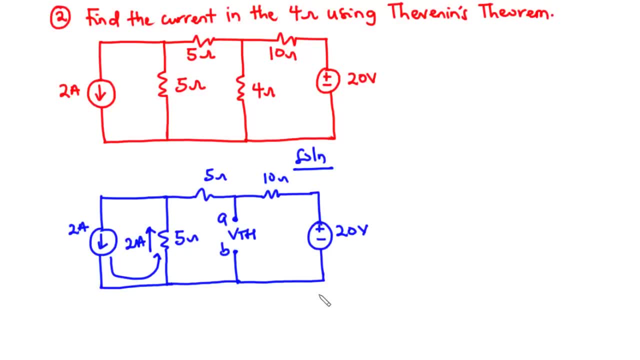 consider this particular loop. So for this loop, this 24 volt source is going to drive current in the anticlockwise direction through this loop. So, considering the conventional flow of current, we have current moving in this direction, that is, the anticlockwise direction, through these three resistors and then 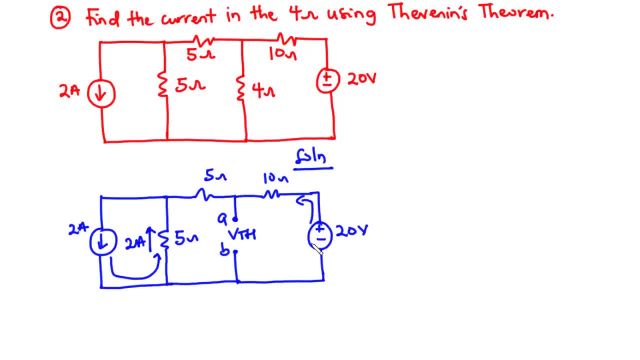 returning to the negative terminal of this voltage source. Now let's call the current driven by this voltage source to be I. So what this primarily means is that we have I flowing through the 10 ohms resistor, the 5 ohms resistor And, at this point, the total current that flows through the 5 ohms. 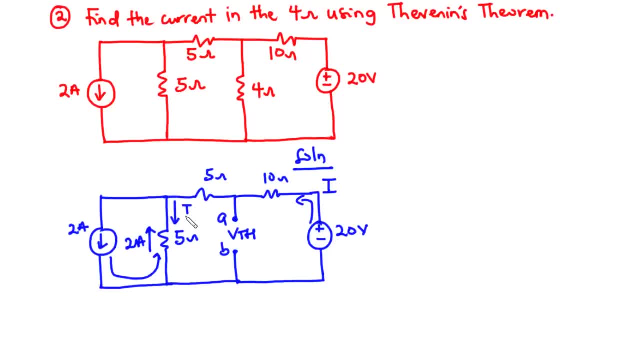 resistor is the value of I minus the 2 amperes current flowing through the 5 ohms resistor. So the total current flowing through the 5 ohms resistor is I minus 2.. Now we have no current flowing through this branch because this is an open circuit, so all the current will like to flow through this. 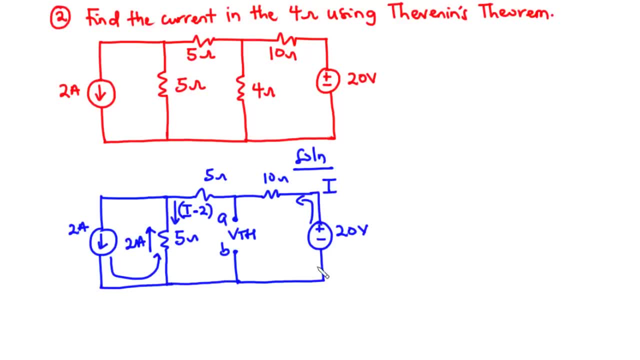 direction and then return to the negative terminal of the voltage source. At this point we can find the value of I. So, considering this loop, we have the voltage source, which is 20 volts, equals the voltage source over the voltage, So in this case we can see that the voltage source is actually constant. 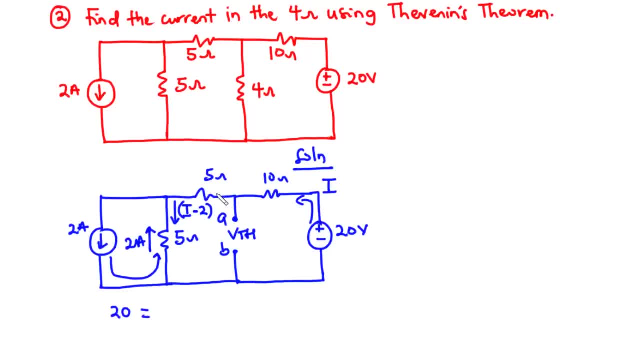 equals the sum of the voltages dropped across the loop. So we have 10 times I plus 5 times I. and then here we have 5 times into bracket I minus 2.. So that is plus 5 into bracket I minus 2.. 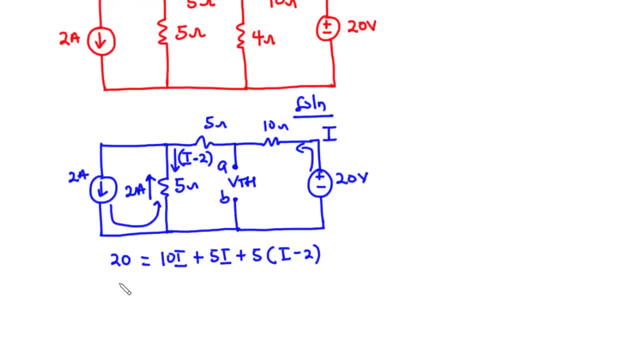 So let's move on, as we want to find the value of I. So we have 20 equals 15I, plus we distribute 5 across, we have 5I minus 10.. So we add these two and then we have 20I, and then we transpose negative 10 to the left. 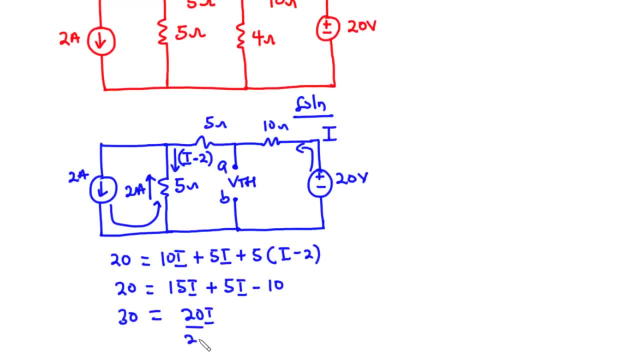 hand side, This becomes 30, and then we divide through by 20 and then we have the value of I to be equal to 3 over 2, which is 1.5 amperes. So this is the value of I, the current, driven by the 20 volts source. 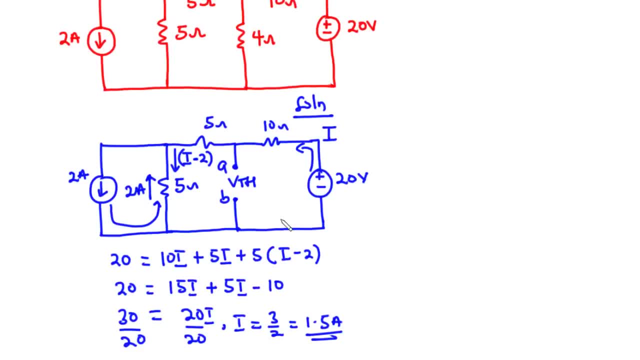 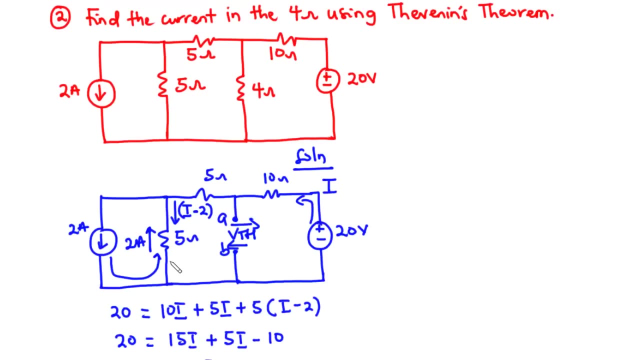 Now, from this we can find the value of Vth, So we can look through the terminal along this direction. we can also view it from that direction. Whichever position you stand, you are going to arrive at the same answer. So let's consider this particular loop. 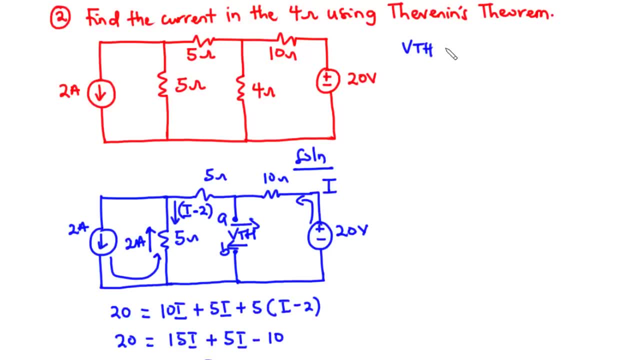 So we have Vth Equals 5 times I, because we have I flowing through this 5 ohms resistor. So that is 5I, and then we are moving in the anticlockwise direction. This is also in the anticlockwise direction, so it remains addition. 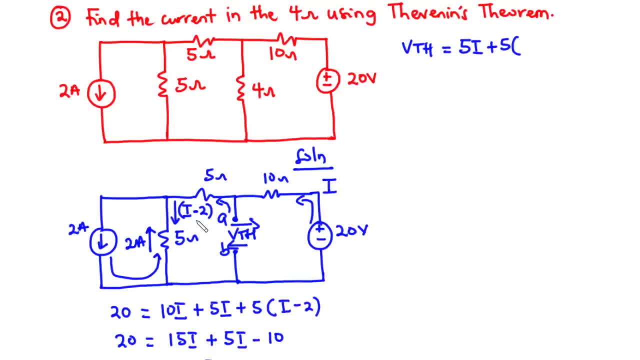 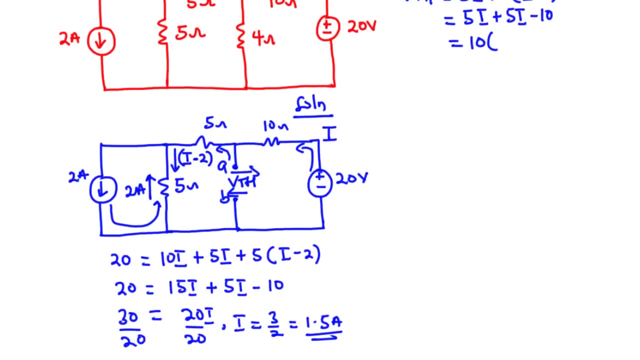 So plus 5 times I minus 2.. So let's simplify. So we have 5I plus 5I minus 10.. 5I plus 5I is 10I, so we have 10. and then we found the value of I to be 1.5.. 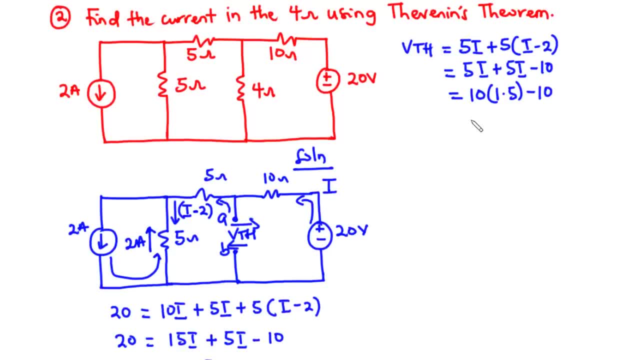 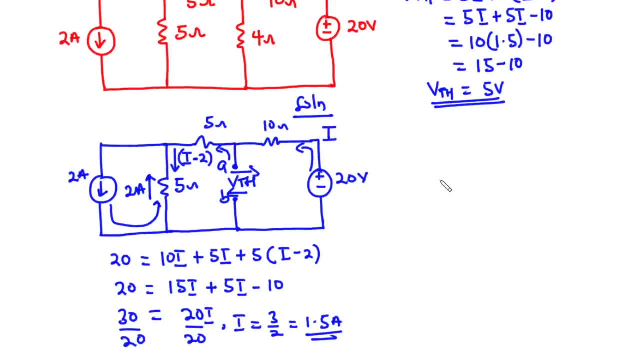 Therefore, we have 10 times 1.5 minus 10, and this is equal to 15 minus 10, and we have the value of Vth to be 5 volts. Therefore, Vth is equal to 5 volts. Now let's find the value of Rth. 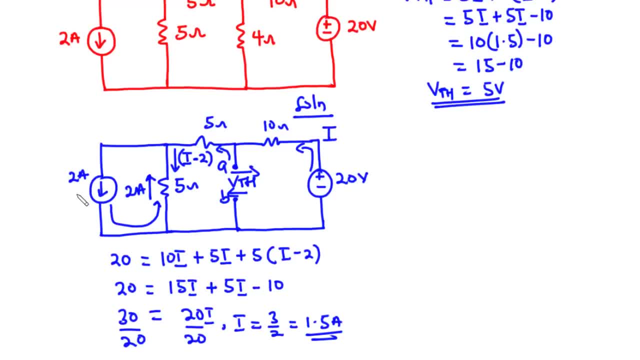 So from this circuit we are going to replace the current source with an open circuit and then short circuit, the voltage source. So this becomes: we have the 5 ohms resistor, we have also this 5 ohms resistor and we have this to be the terminal AB. 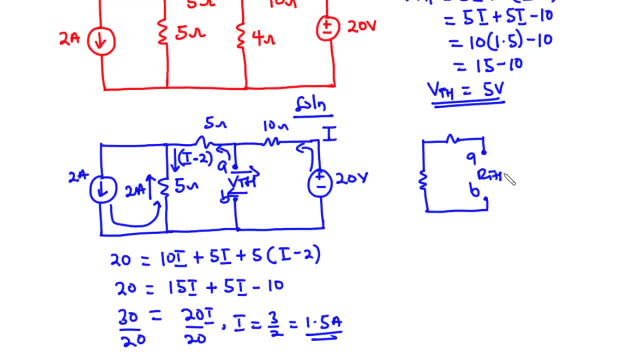 5V, 5V, 5V, 5V, 5V. We have this 10 ohms resistor and then we short circuit the voltage source, So we have 10,, 5 and then 5.. Now, assuming that we have a voltage source here, then at this point we have the current. 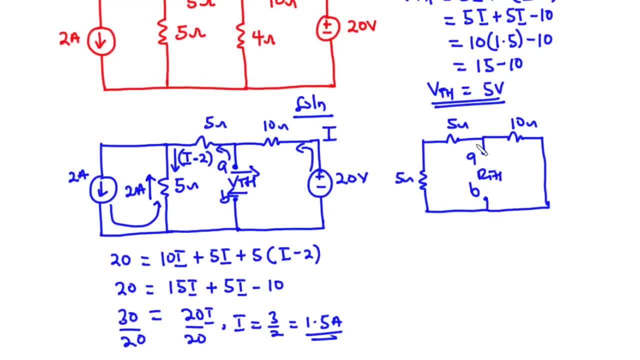 going to divide, So we have part of the current flowing through this direction and then the other part also flowing through that direction. Now the current that flows through this 5 ohms resistor will be the same current that flows through this 5 ohms resistor, which clearly means that these two resistors are connected. 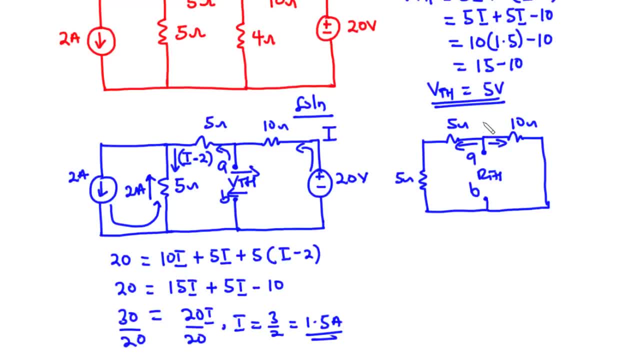 in series and their combination is connected in parallel with this 10 ohms resistor. Therefore we have Rth to be equal to 5 plus 5, that is for the two series resistors in parallel with the 10 ohms resistor, So this becomes 10.. 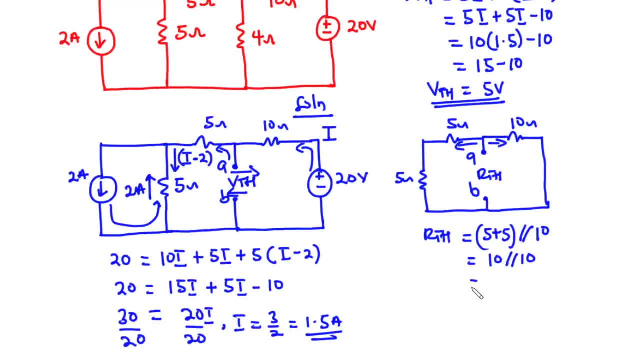 Parallel 10.. And when two resistors of the same value are parallel to each other, then the resultant is half their value. So 10 parallel 10 is equal to 5.. So we have Rth to be equal to 5.. 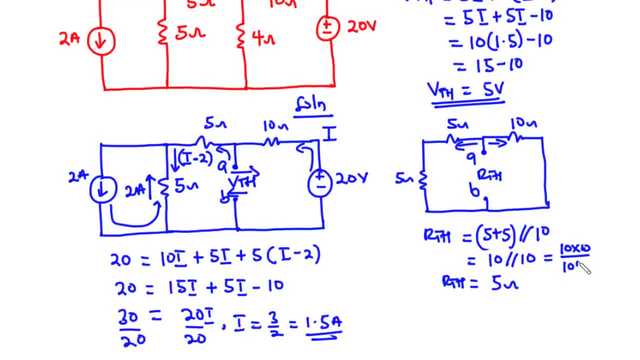 If you have 10 times 10, divided by 10, plus 10.. 10 times 10 is 100, divided by 20 is 5.. So we have Rth to be 5.. Now let's find The value of the current flowing through the 4 ohms resistor.